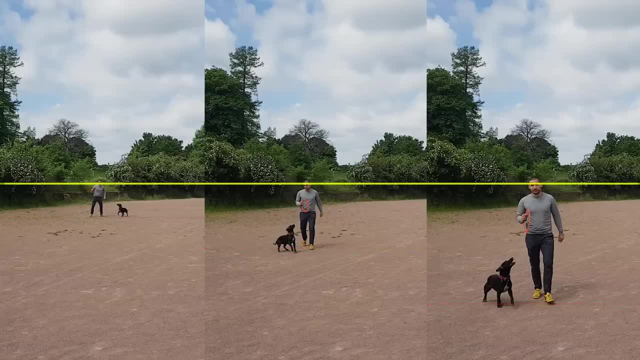 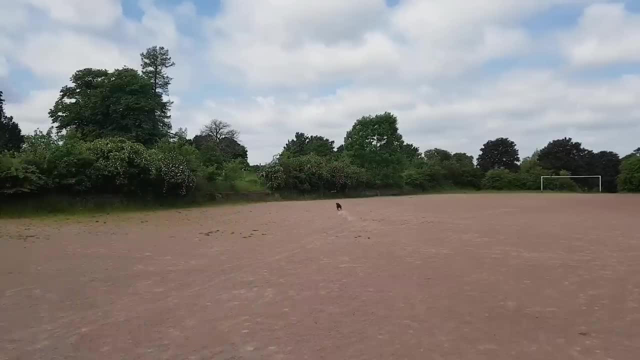 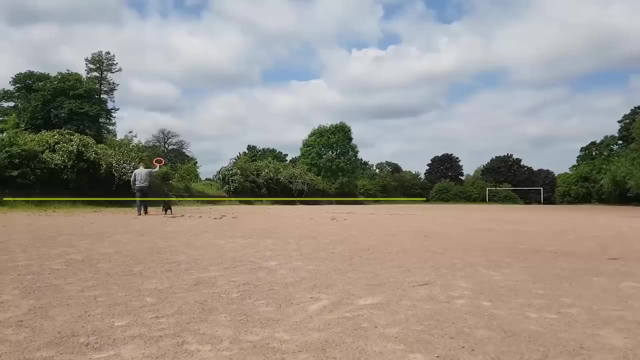 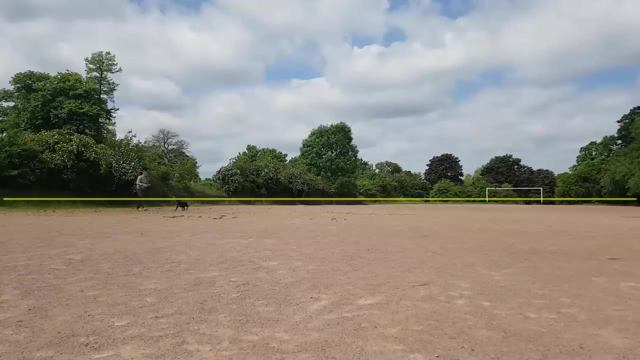 so they're below the horizon or the eye level line, and they move further away from it as we get closer. this time i set the camera down low, so now we're seeing maggie's eye level. my eyes are above her eye level, so they're above the horizon line. now we're far from the camera, so my eyes 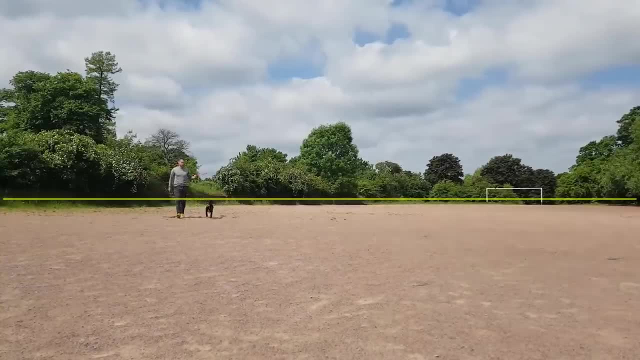 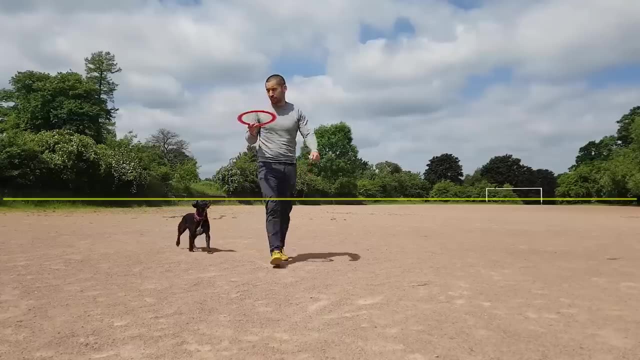 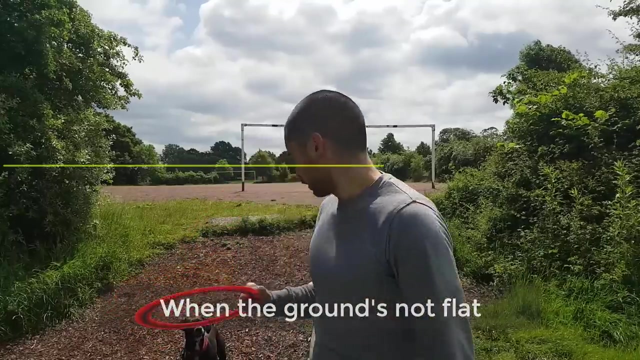 aren't too far from the eye level line, but as we move towards the camera they move further and further away from it. maggie's eyes are staying on that line because we're seeing maggie's eye level now. now the camera is back at my eye level and i'm gonna move up this hill and that has the same. 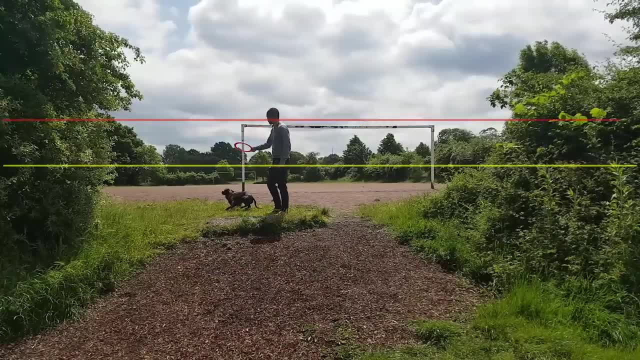 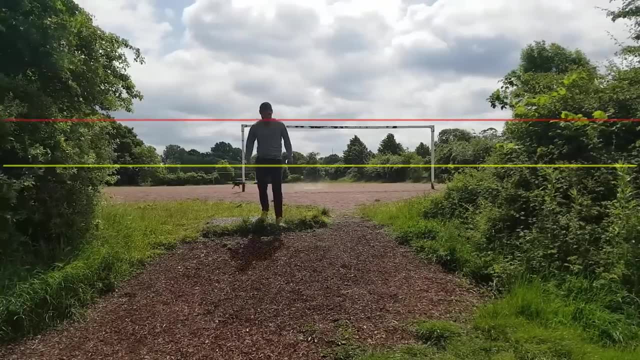 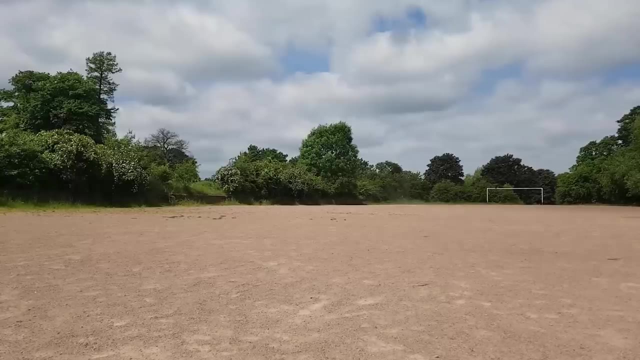 effect as if i was becoming taller. my eye level goes up, but the camera level stays the same, so it doesn't stay in line with my eyes and my eyes move up in the frame. so next time your friend is walking towards you or you throw a frisbee for a dog and they run back to you notice how their eyes are moving. 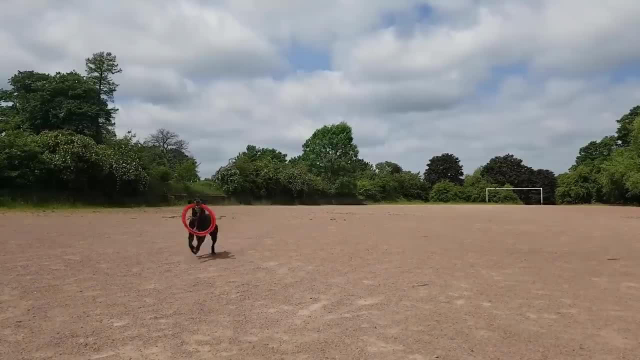 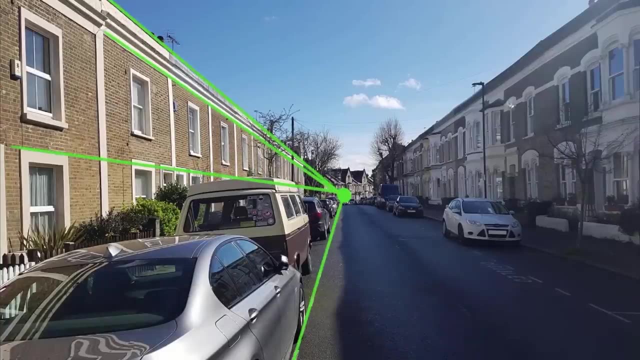 are they going up or down relative to your eye level? remember when we looked at this street and noticed how all the lines- because they're pretty parallel- they all end up at the same vanishing point and that was pretty much on the horizon line. and then we looked at these cereal boxes and noticed that they had different vanishing points. 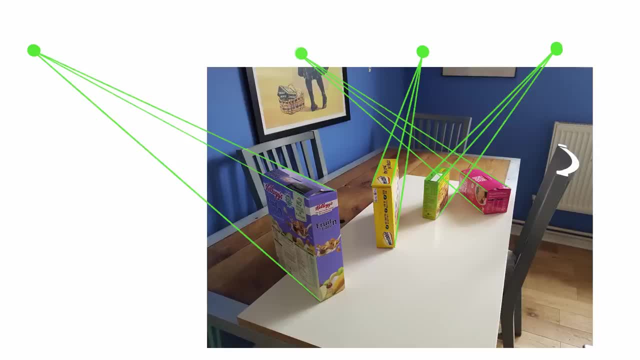 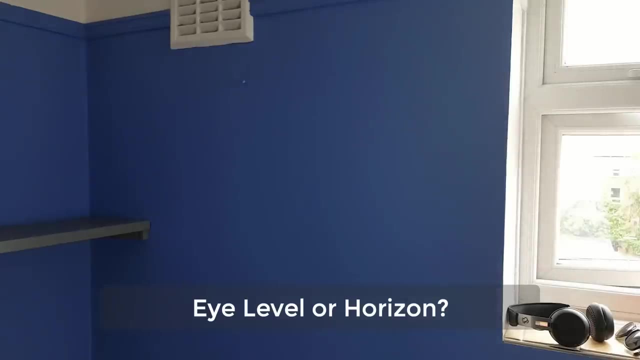 because they weren't parallel. they were all pointing in different directions, but look, the vanishing points were all on the same line, and that is the eye level line, or the horizon line, in this case the level of the camera. so that's really awesome. i think it can be confusing when you talk about the horizon line this way. sometimes you might. 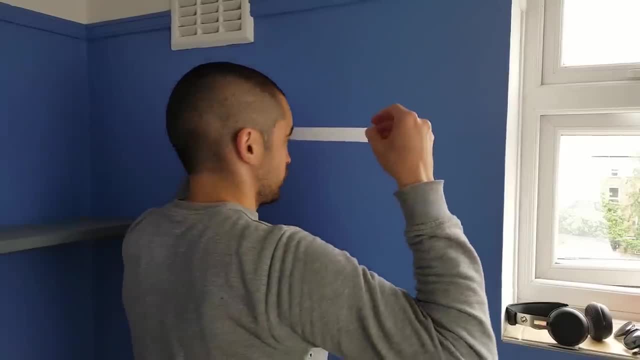 have all sorts of things in the way stopping you from seeing the proper horizon line, like some buildings or just walking around the area or any kind of nice forgotten style in the road or even the see the horizon line. you might see the car and go into the return lane and some buildings or just 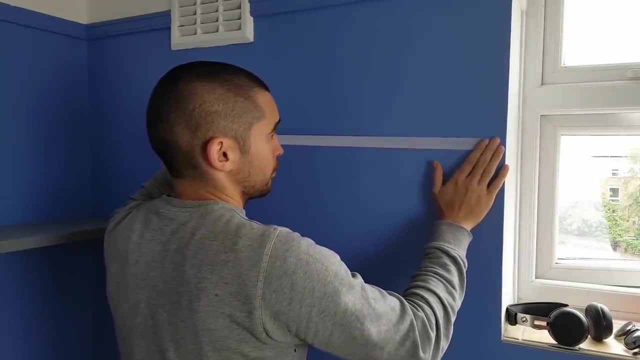 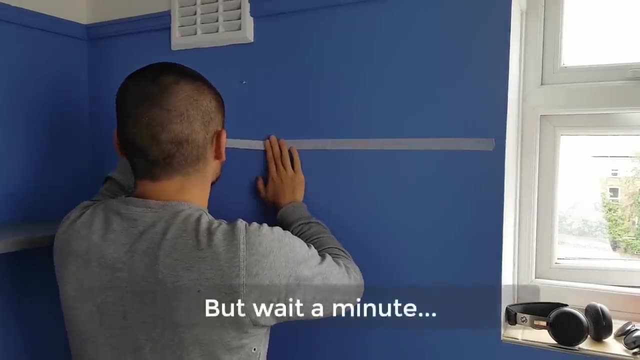 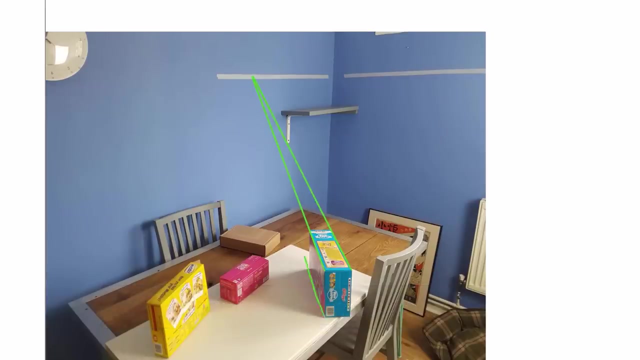 walls if you're inside. if you went around the wall with some masking tape at your eye level, as you do, that would be the same level as the horizon line. okay, so up until here i'm feeling pretty good, maybe even a little bit smug. i feel like i'm 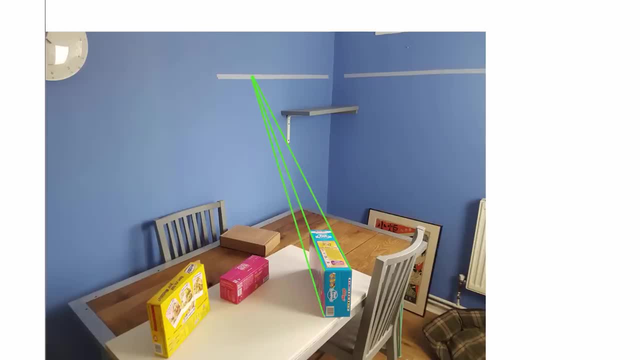 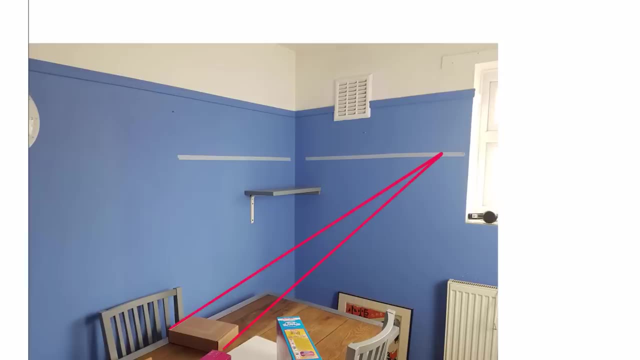 understanding perspective. i'm walking around town, i'm having my breakfast, i'm getting better and better at seeing this eye level stuff all the time. but wait, what's this? when i open the lid of this box, the lines of the lid are not converging to a point on the horizon line anymore, or the eye level. 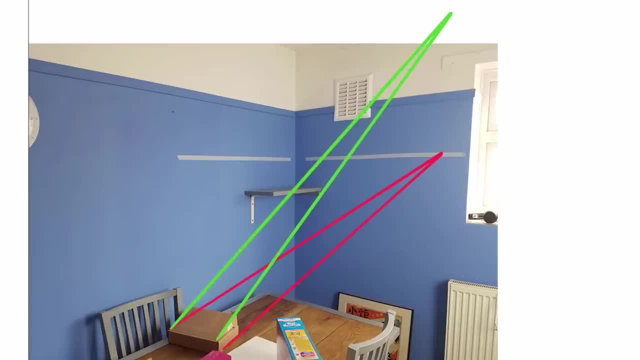 line. this is one of the things that i think often isn't explained and i've found confusing, because it's really nice and neat when everything goes to a point on the horizon, but here's the big thing: it's only the lines of things that are converging to a point on the horizon. 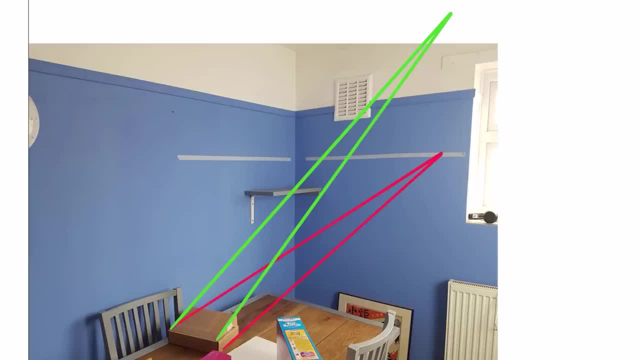 that are parallel to the ground, that are going to converge to the horizon line. if something tilts- so it's not parallel to the ground- the vanishing point could be above or below the horizon, so now it feels like chaos. i thought everything was going to go to the horizon line, but it's okay. 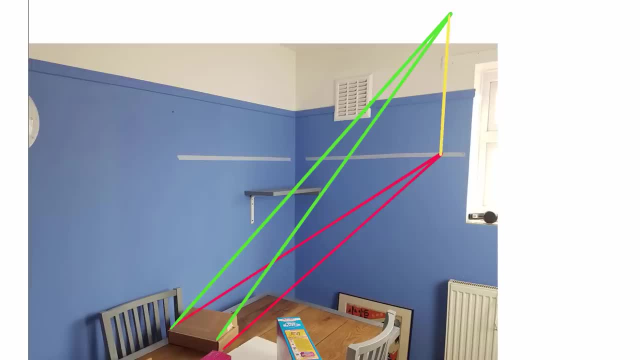 the point it goes to will be directly above or below where the vanishing point would be when it was parallel to the ground. so it's just moving straight up and down and it's not converging to the horizon line. it's just moving up or straight down, depending on how it's tilting. 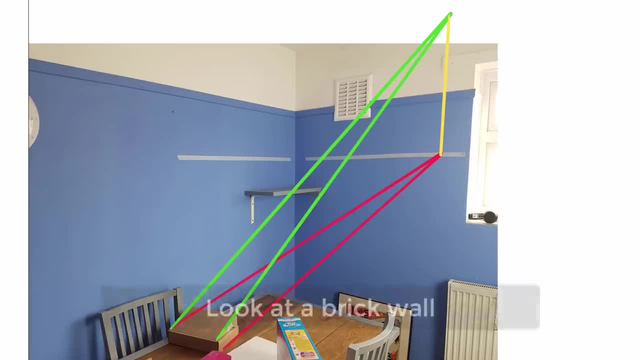 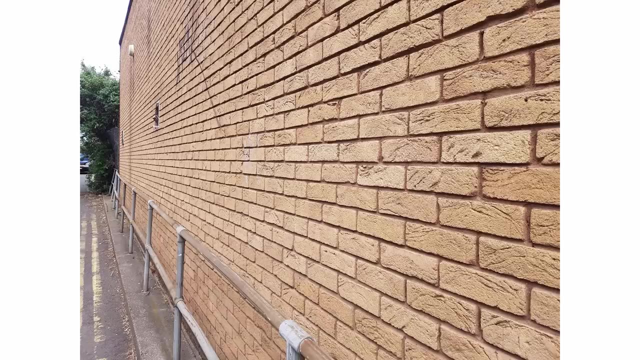 that doesn't feel too bad. i think i can handle that. rows of bricks are usually parallel to the ground, so when you're walking next to a wall you can see. the lines of bricks that are below your eye level will be angled upwards the ones that are at your. 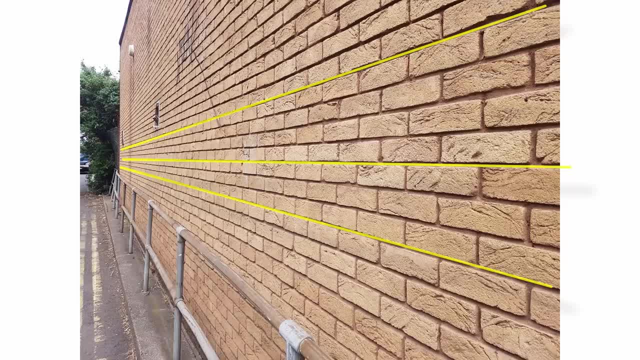 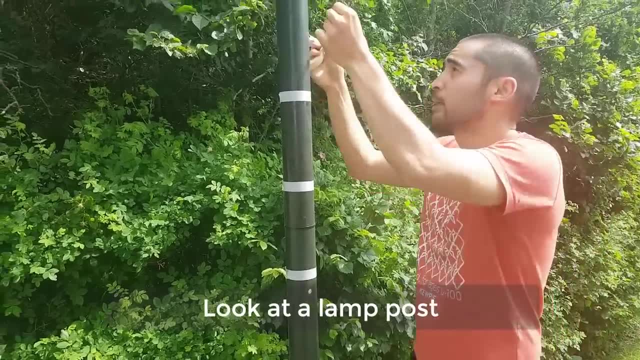 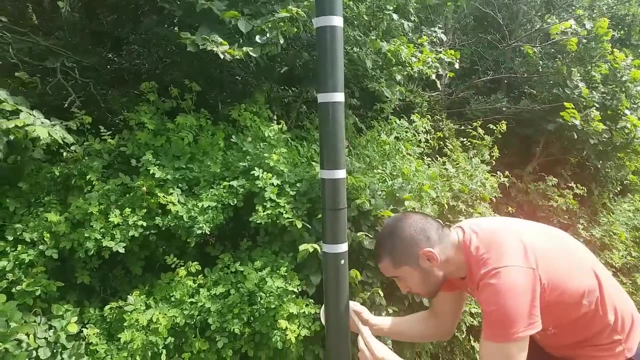 eye level will be straight across and the ones that are above your eye level will be angled downwards, converging down to the eye level all right. so this is where i reveal that this series is really an elaborate ruse designed to get people to think that you've gone bonkers, because i'm going to ask you to just look at a 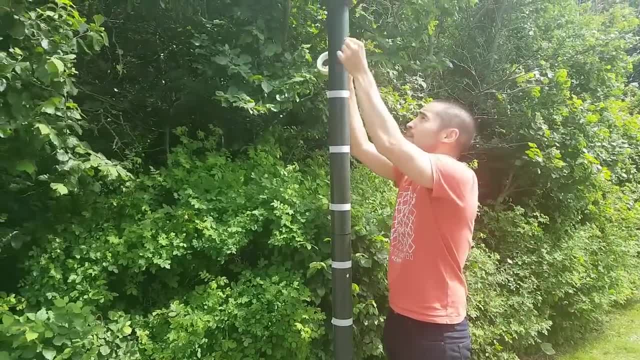 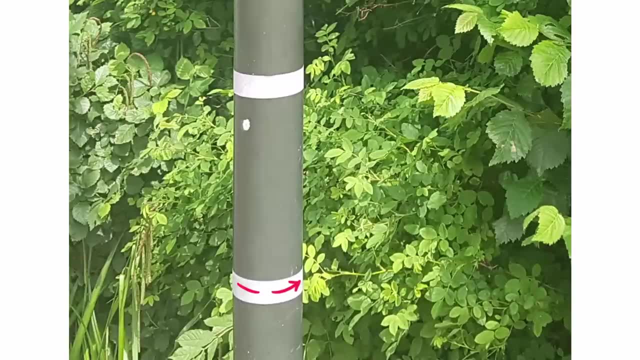 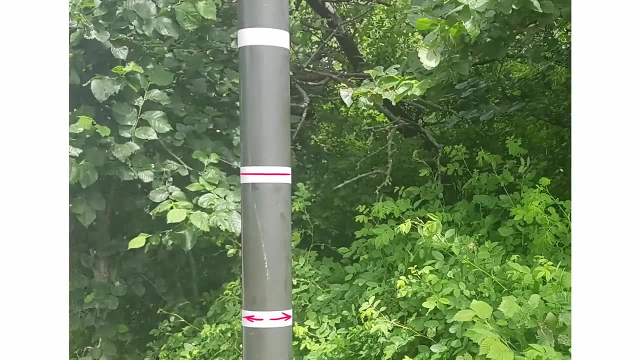 lamp post next time you pass one and then imagine there are lines going around it. below your eye level they'll be curving upwards and at your eye level the line will be straight, and above your eye level it'll curve the other way. and that's really because the lamp post is.